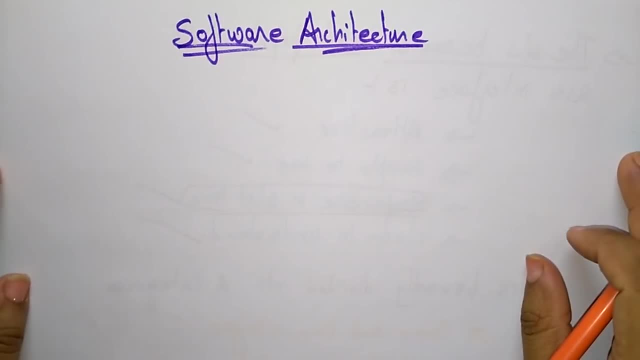 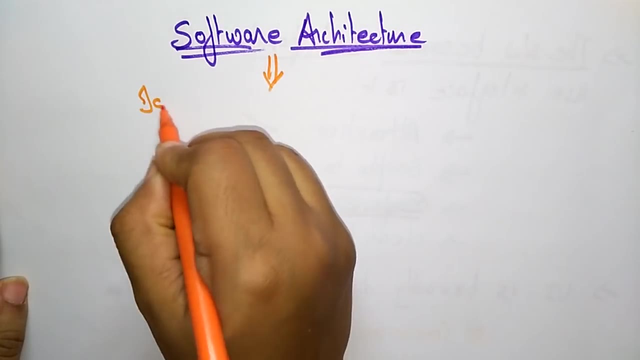 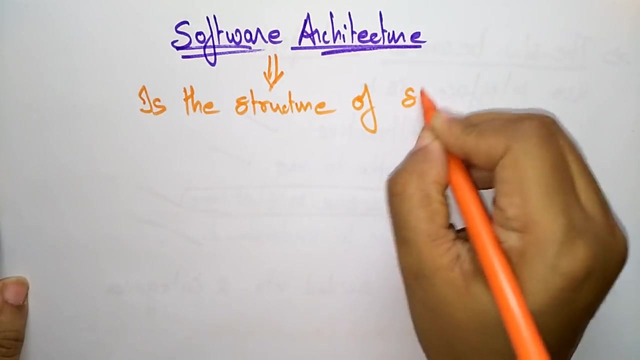 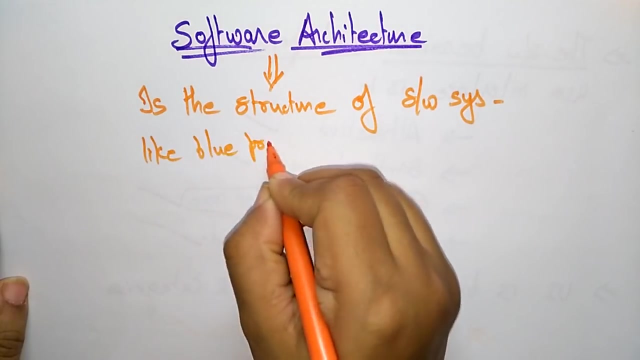 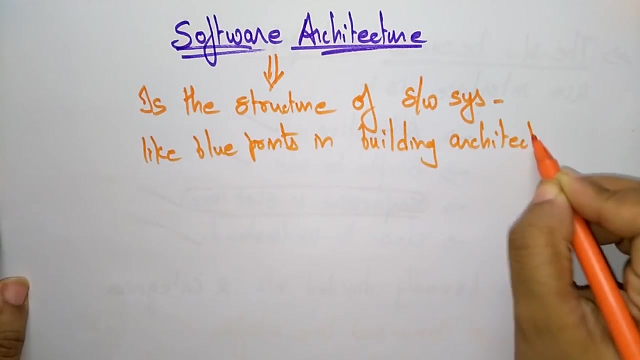 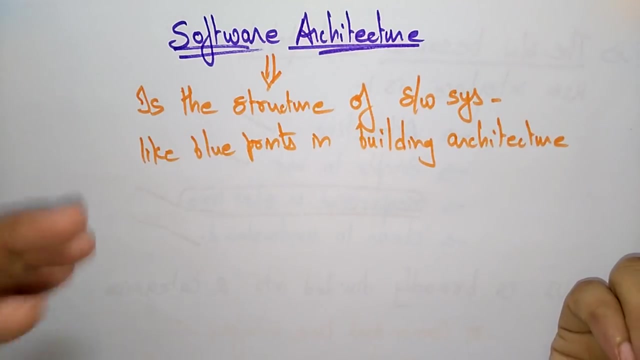 Hi students. coming to the next topic in the subject, software engineering, was software architecture. So what is a software architecture? A software architecture is the structure of software systems, like blueprints in building architecture, Suppose. let us take a building architecture. If you want to build any, if you want to construct any building first you need some architecture blueprint. So before starting the work they have to present everything in the paper So that you call it as a blueprint. In the same way, if you want to develop any software, if you want to develop any apps, first you require some blueprints, So that blueprint you call it as a software architecture. 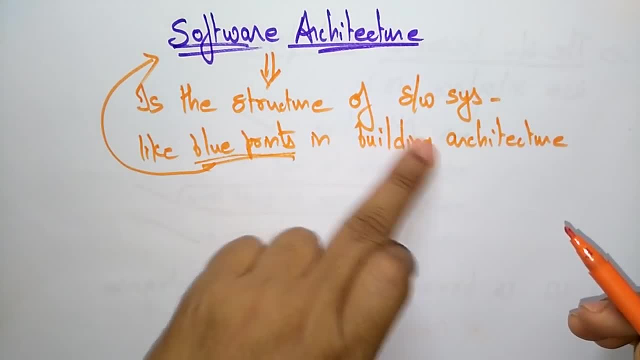 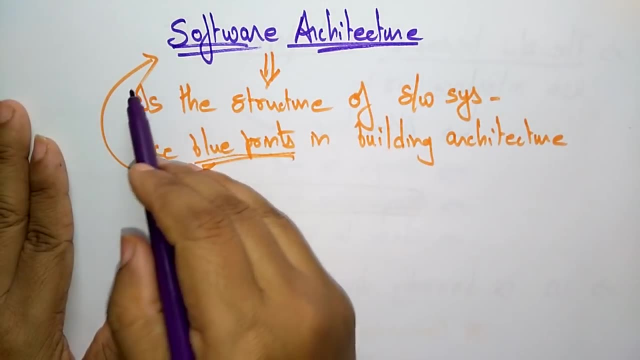 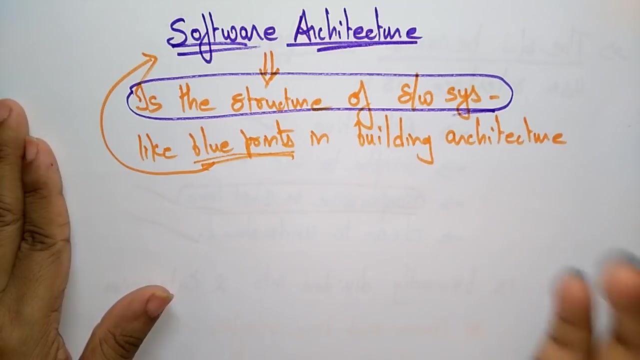 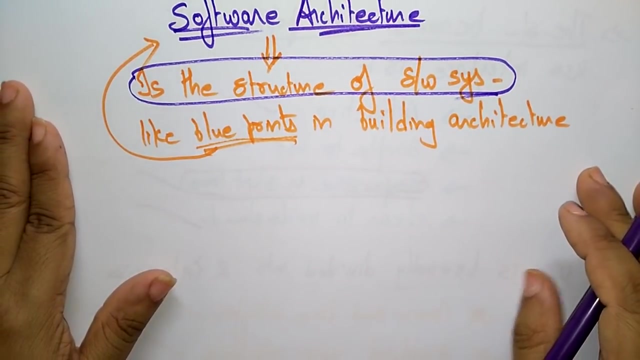 A software architecture is a structure of software systems, like blueprint in building architecture. So the main definition for the software architecture is the structure of software systems. So whatever the software systems that you are using, so that software system is represented in the form of a structure, That structure you call it as a software architecture. 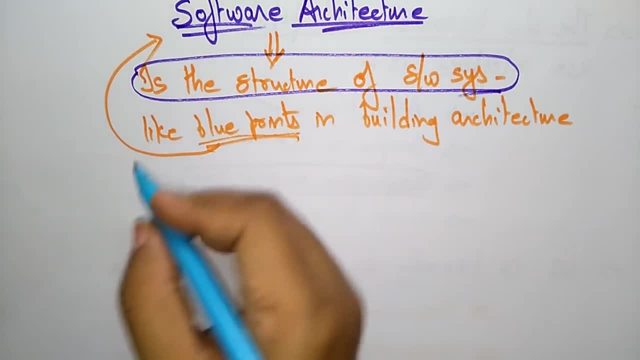 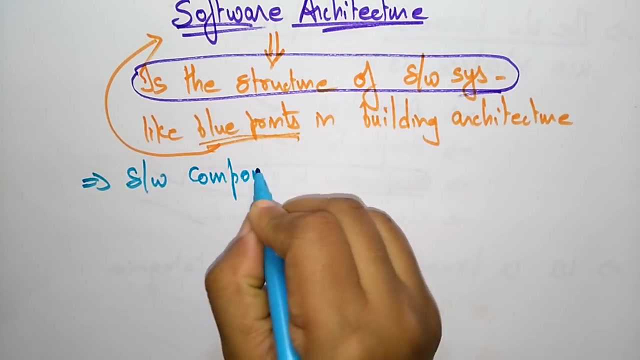 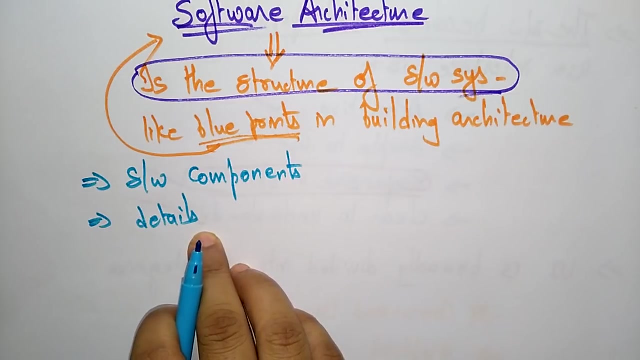 So this software architecture consists of some software components. If you want to develop, if you want to build any software architecture- either it is in software or it is in the hardware means the buildings. whatever it may be- you need some software components, details, details about data structures and algorithms that are hidden in that software. So you need software components and the details regarding data structures and algorithms. 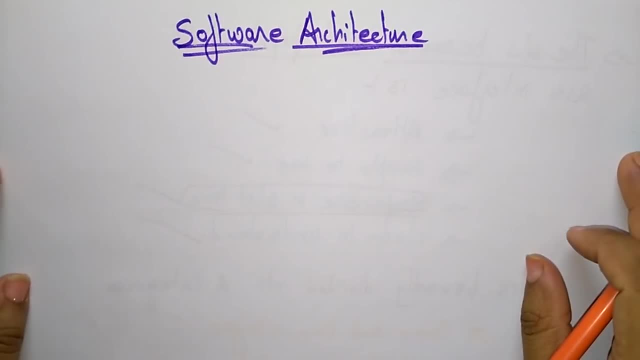 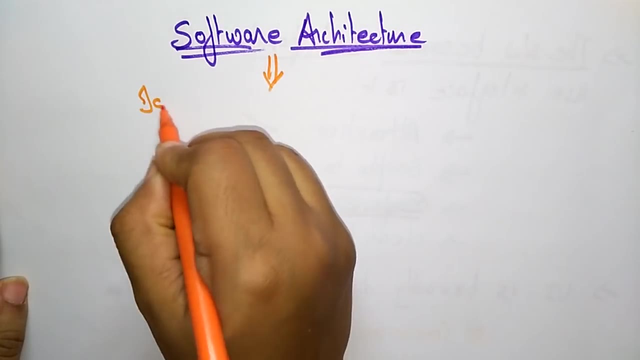 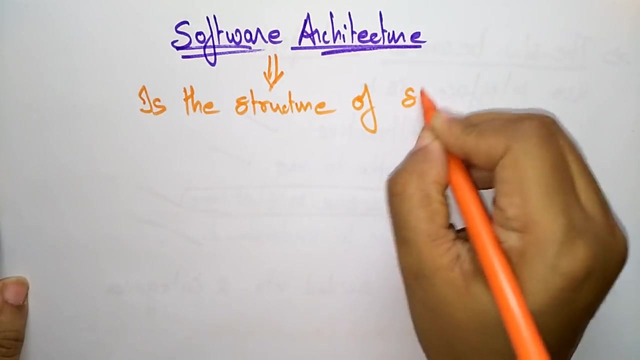 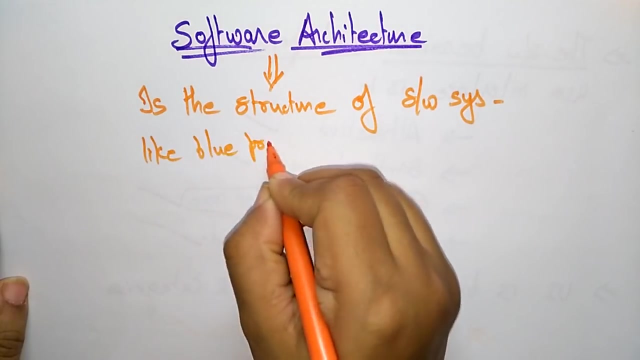 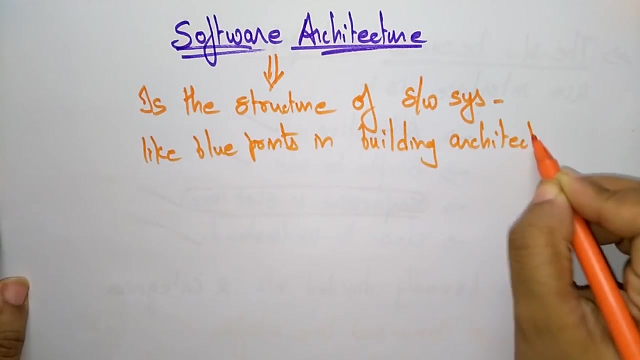 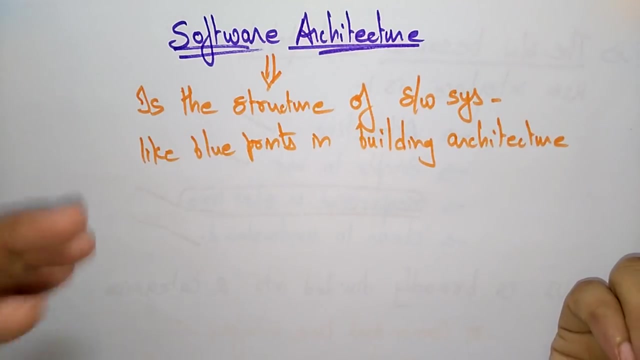 Hi students. coming to the next topic in the subject, software engineering, was software architecture. So what is a software architecture? A software architecture is the structure of software systems, like blueprints in building architecture, Suppose. let us take a building architecture. If you want to build any, if you want to construct any building first you need some architecture blueprint. So before starting the work they have to present everything in the paper So that you call it as a blueprint. In the same way, if you want to develop any software, if you want to develop any apps, first you require some blueprints, So that blueprint you call it as a software architecture. 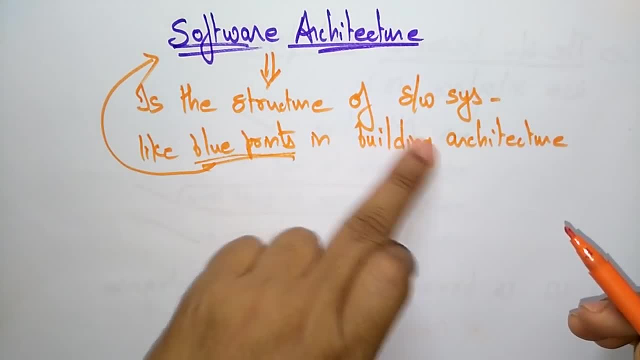 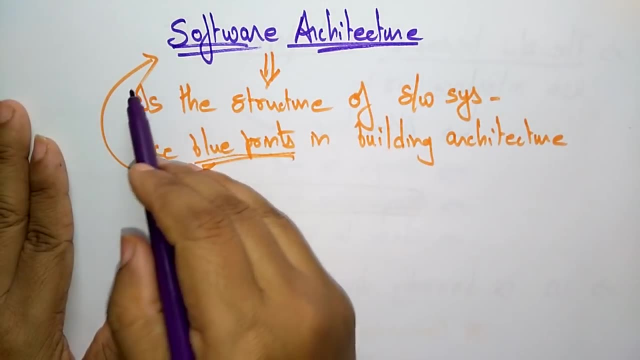 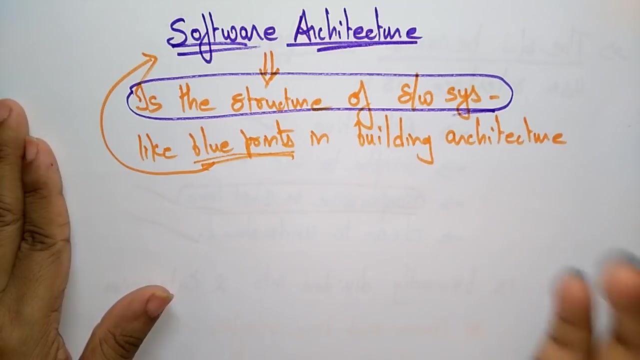 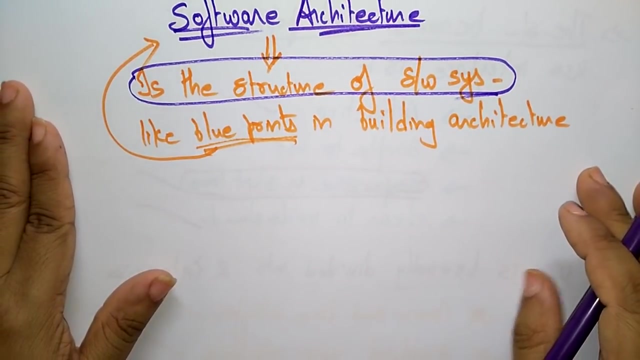 A software architecture is a structure of software systems, like blueprint in building architecture. So the main definition for the software architecture is the structure of software systems. So whatever the software systems that you are using, so that software system is represented in the form of a structure, That structure you call it as a software architecture. 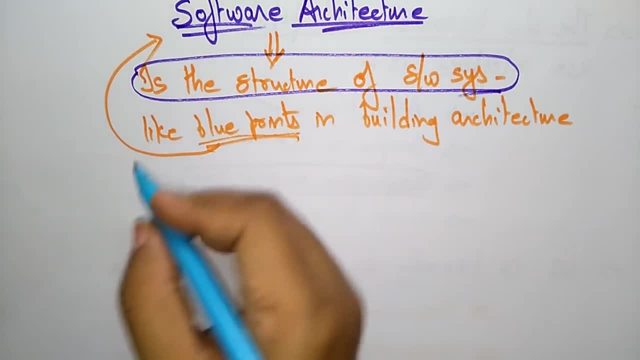 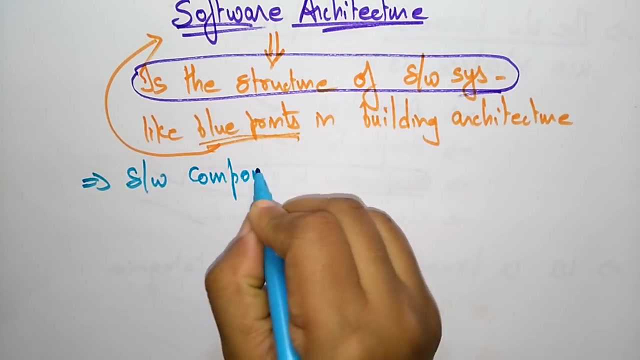 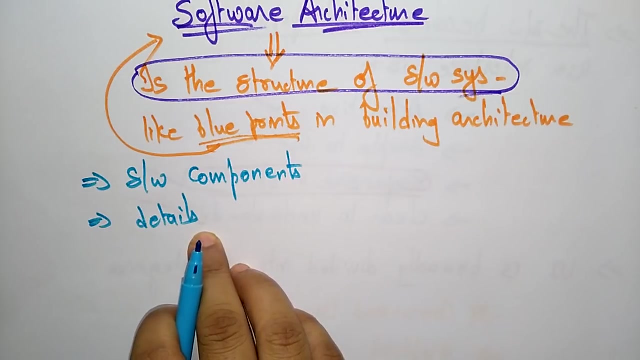 So this software architecture consists of some software components. If you want to develop, if you want to build any software architecture- either it is in software or it is in the hardware means the buildings. whatever it may be- you need some software components, details, details about data structures and algorithms that are hidden in that software. So you need software components and the details regarding data structures and algorithms. 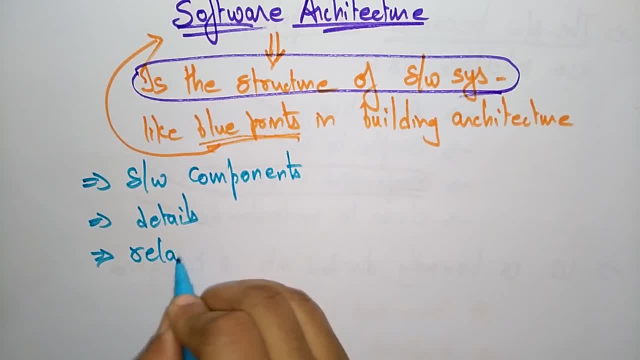 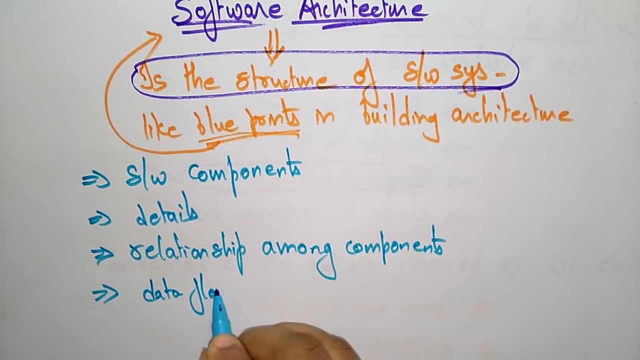 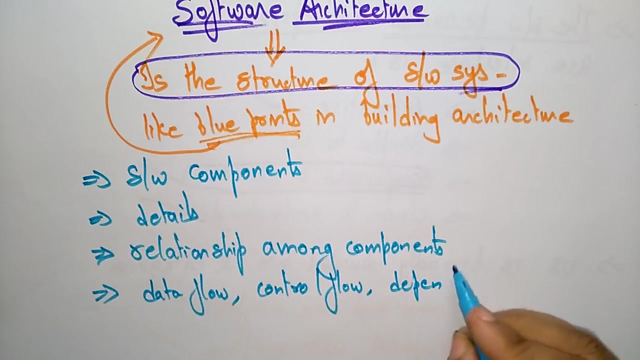 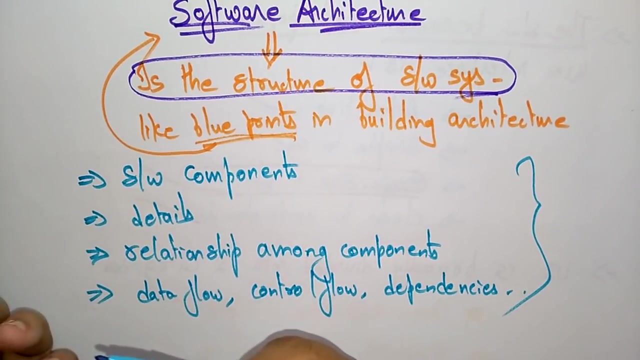 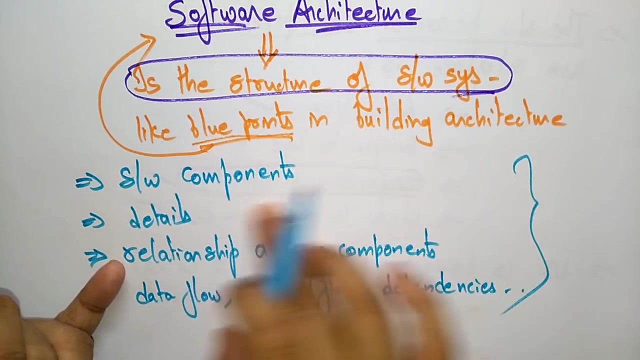 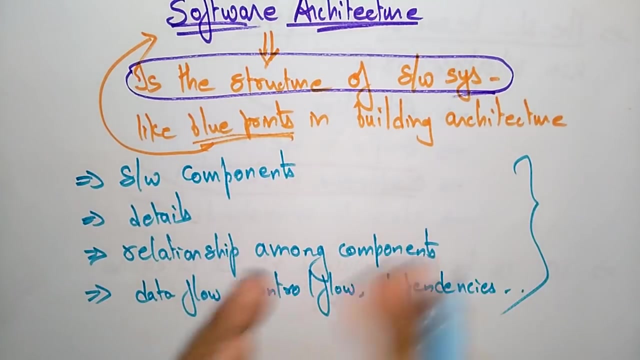 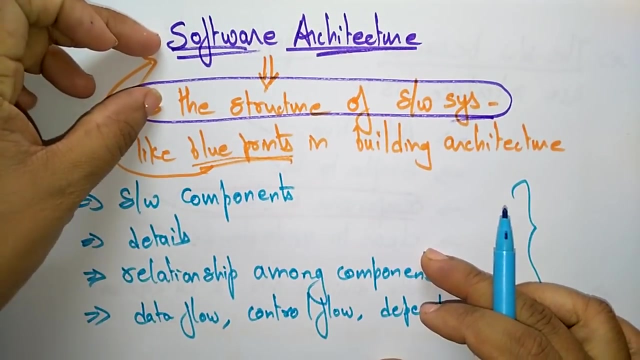 And relationships among the components, Relationship among components and the relations like. if you know the relations like data flow, control flow, dependencies, dependencies- Okay, So if you know all these things regarding the software, So whatever the software you are going to develop, So if you know the software components that are used in that software and the details regarding the data structures and the algorithms that are hidden in the software and the relationships among the different components that are present in the software and the data flow from one component to another component, and what is the control flow and what are the dependencies- either this component is dependent on this or like that- If you know all the details, then you can develop a software architecture. 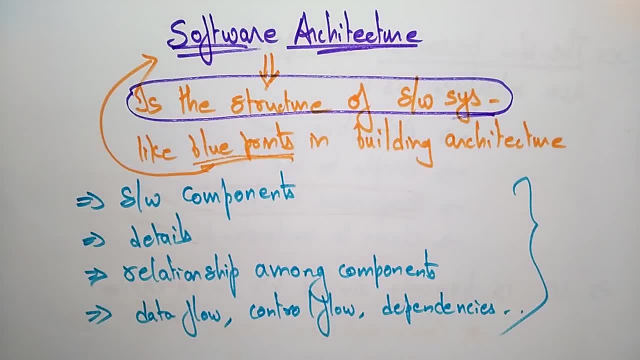 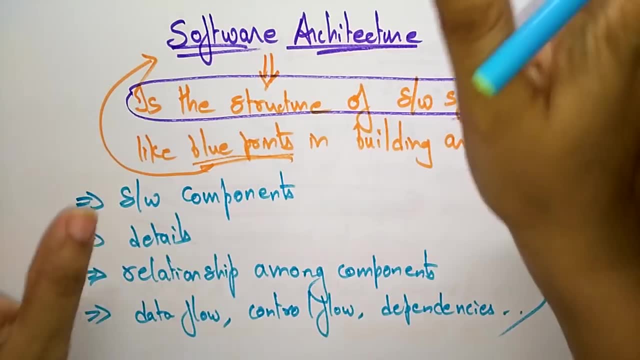 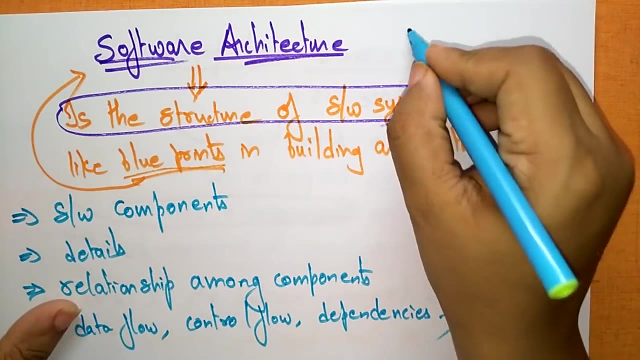 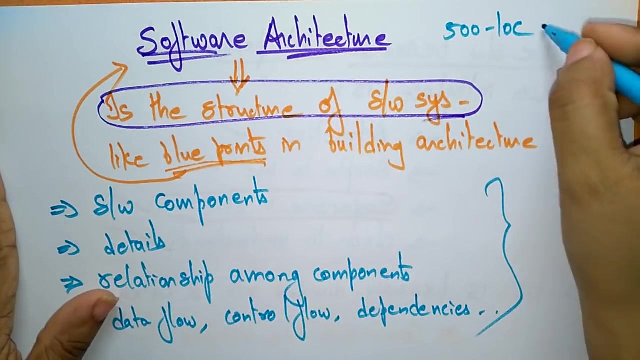 Okay, so actually why we need a software architecture. means: is it necessary to draw a software architecture for every software? No, it's not compulsory. means: if your software is less lines of code- suppose if it is around 500 lines of code- okay, if your software project is around 500 lines of code is just write it, no need of architecture. 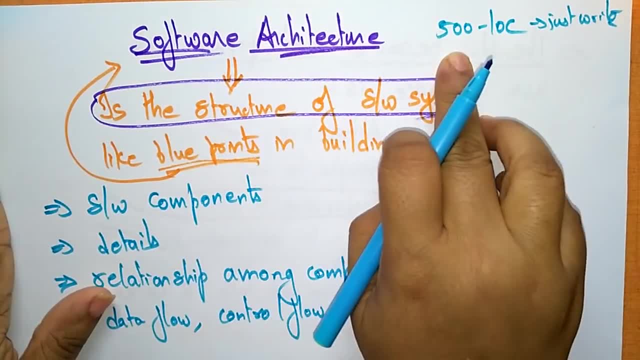 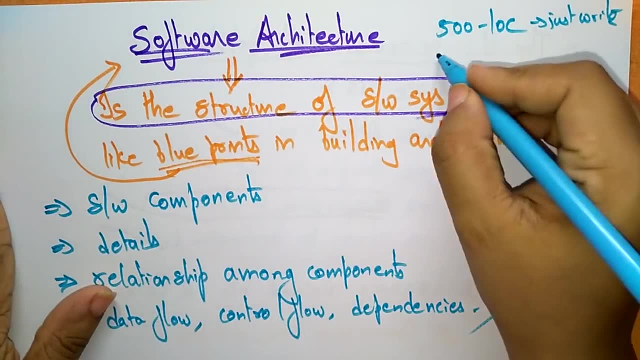 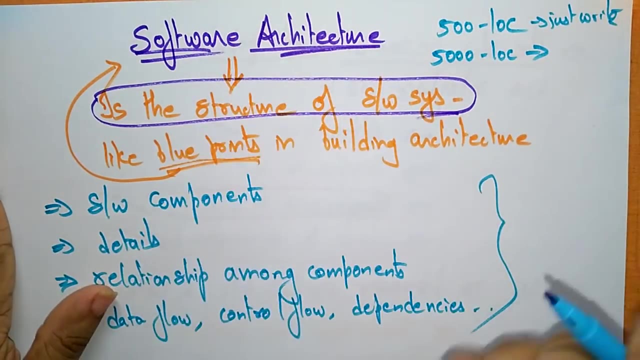 Okay, software software that you are going to develop is just 500 lines of code, just right. don't prepare the software architecture. suppose it is 5000 lines of code further. also, you no need, don't require the software architecture, just use the classes, class diagrams. so with the class. 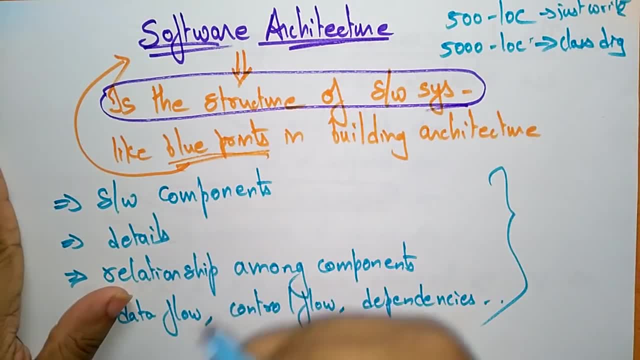 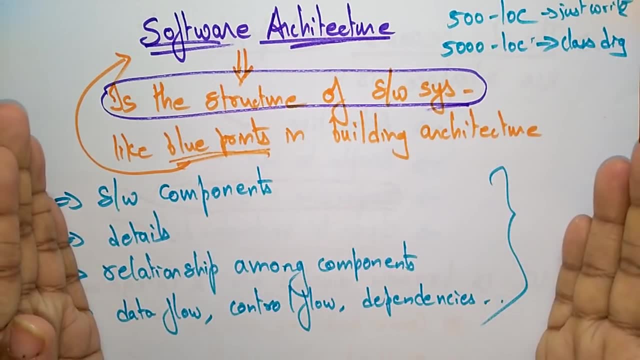 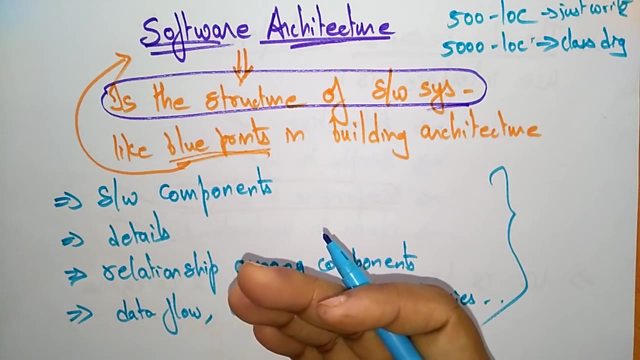 diagrams you can identify the flow from which component to which component the data is transferring and which component is depends upon which component and which component is going to control the other component. so here the components are nothing but the functions that are used in the program. okay, or you call it as a modules, components, modules, functions, everything. everything is same. 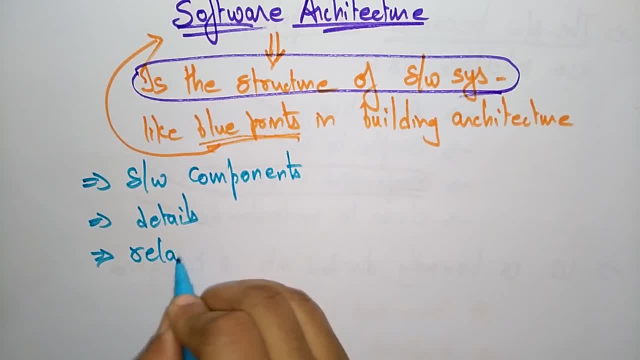 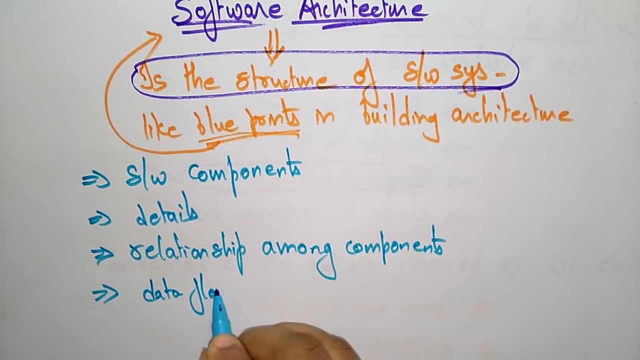 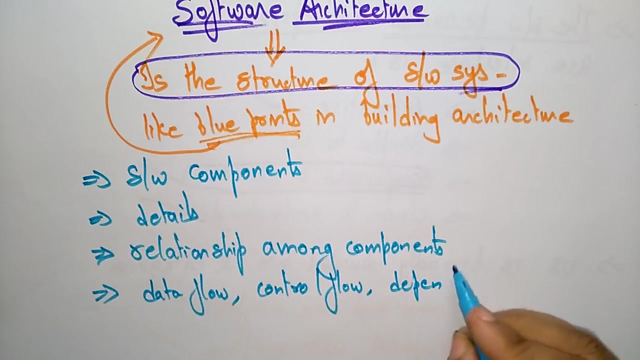 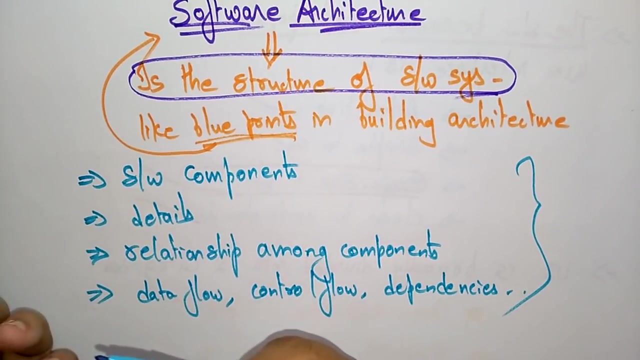 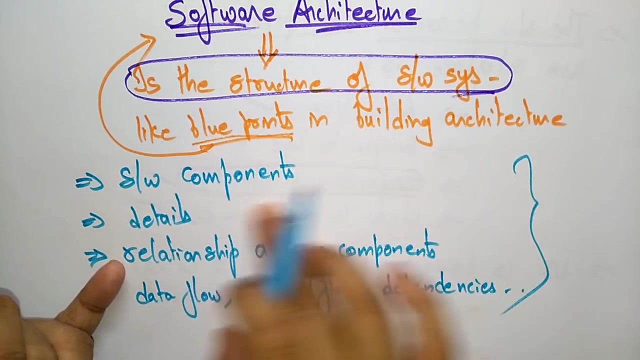 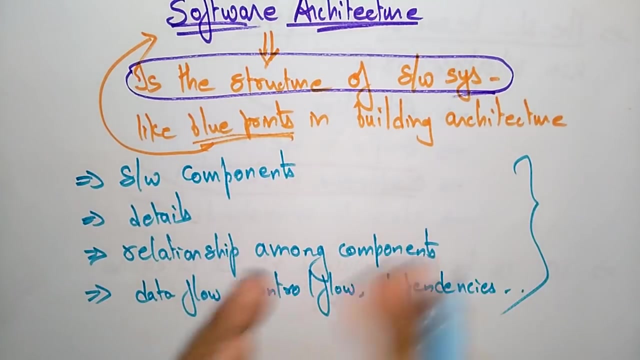 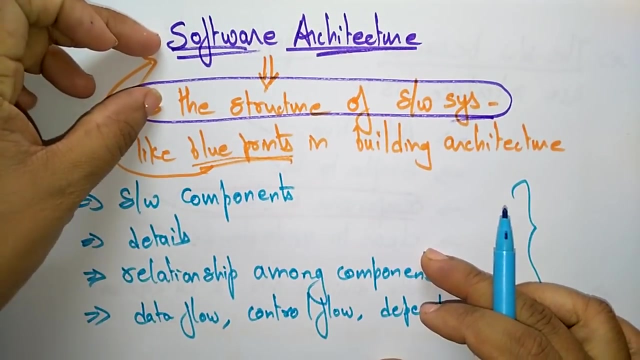 And relationships among the components, Relationship among components and the relations like. if you know the relations like data flow, control flow, dependencies, dependencies- Okay, So if you know all these things regarding the software, So whatever the software you are going to develop, So if you know the software components that are used in that software and the details regarding the data structures and the algorithms that are hidden in the software and the relationships among the different components that are present in the software and the data flow from one component to another component, and what is the control flow and what are the dependencies- either this component is dependent on this or like that- If you know all the details, then you can develop a software architecture. 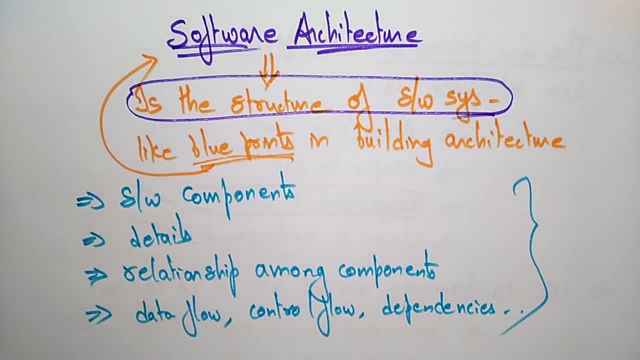 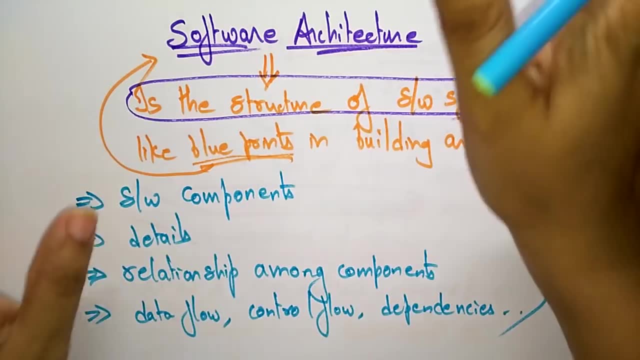 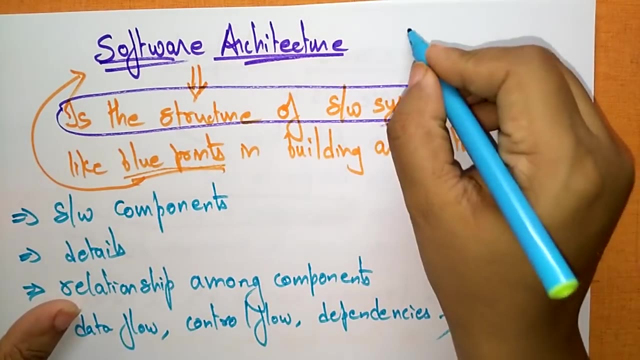 Okay, So actually, why we need a software architecture. means: is it necessary to draw a software architecture for every software? No, it's not compulsory. means: if your software is a less lines of code, Suppose if it is around 500 lines of code. 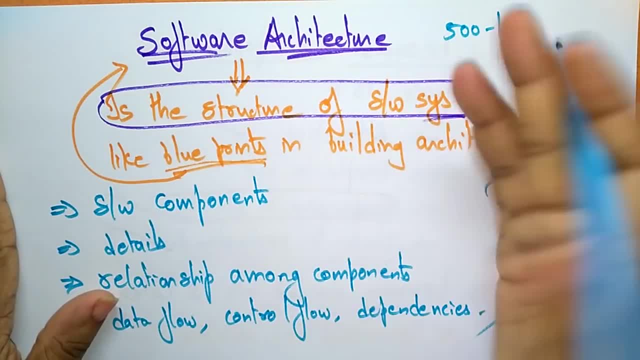 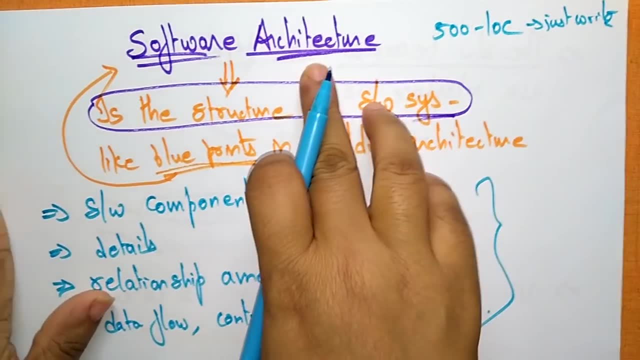 Okay, If your software project is around a 500 lines of code is, just write it, No need of architecture. Okay, If you are. If your software software that you are going to develop is just 500 lines of code, Just right. 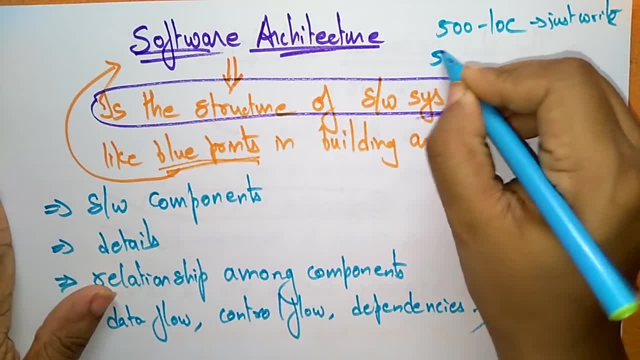 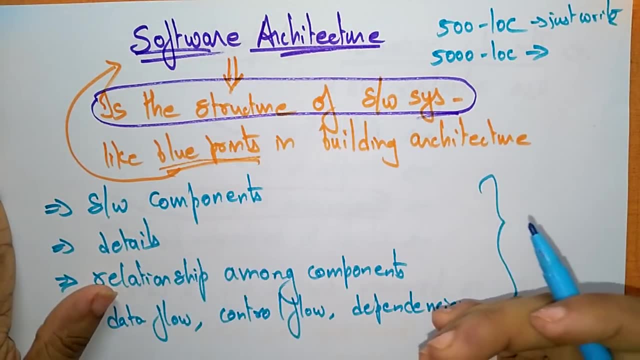 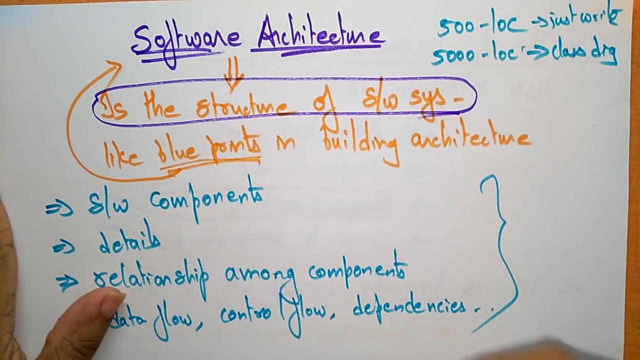 Don't prepare the software architecture. Suppose it is 5000 lines of code Further. also, you don't need, don't require the software architecture, Just use the classes, class diagrams. So with the class diagrams you can identify the flow, from which component to which component the data is transferring and which component is depends upon which component. 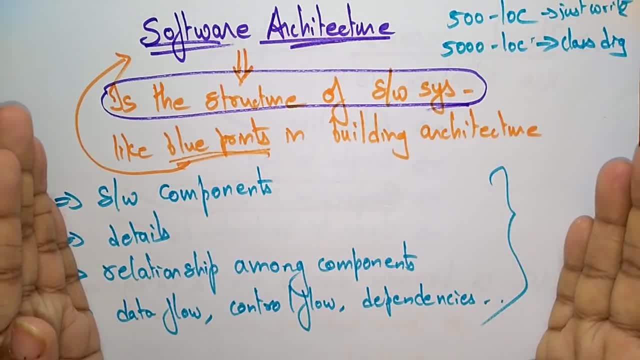 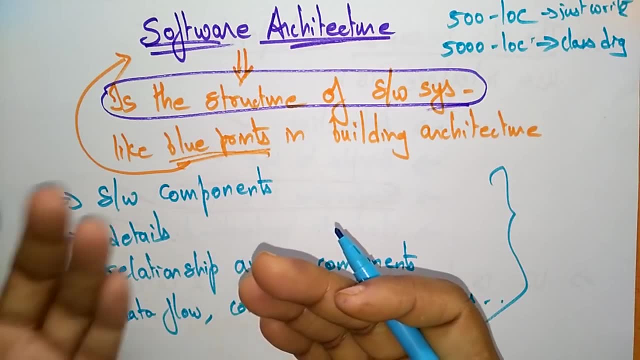 And which component is going to control the other component? So here the components are nothing but the functions that are used in the program. Okay, Or you call it as a modules, components, modules, functions, everything. Everything is same, Okay. 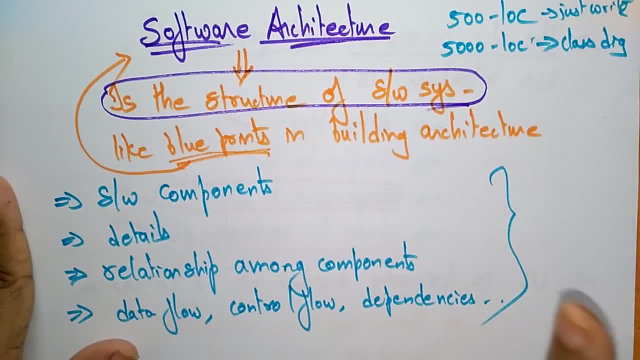 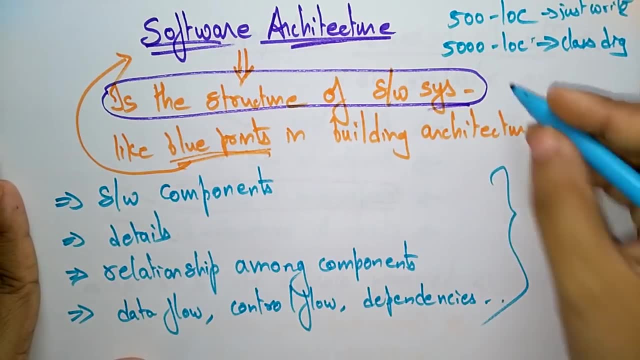 So if it is 5000 lines of code, better go for the class diagram. It is not that much of complicated for these lines of code writing the class diagram. Suppose if it is more than 5000.. Okay, Then the problem will rise. 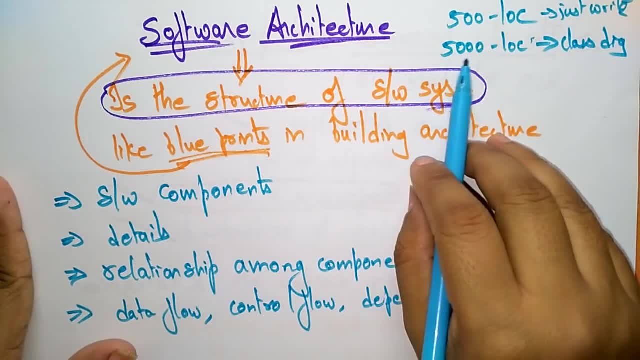 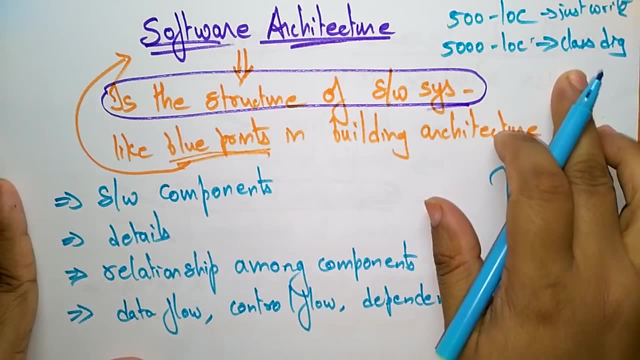 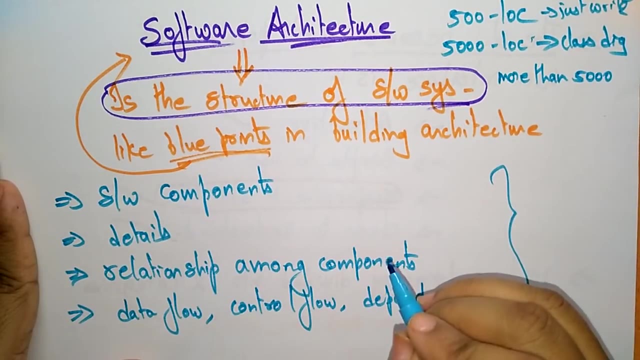 okay, so if it is 5000 lines of code, better go for the class diagram. it is not that much of complicated for for these lines of code, writing the class diagram, suppose if it is more than 5,000, then the problem will rise. so if, in this case, if your program is more, 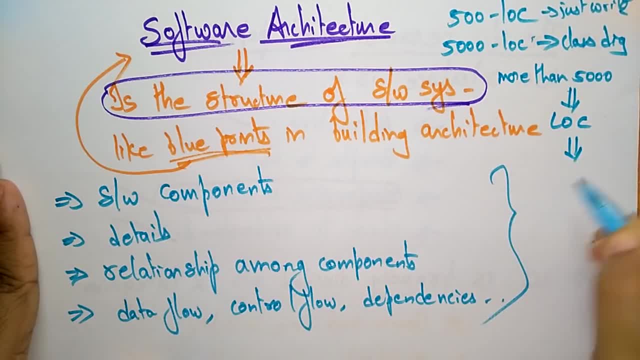 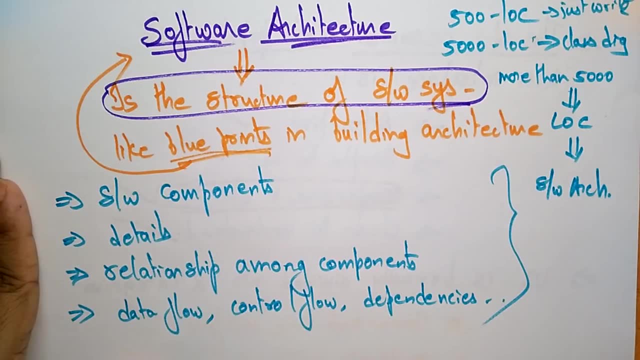 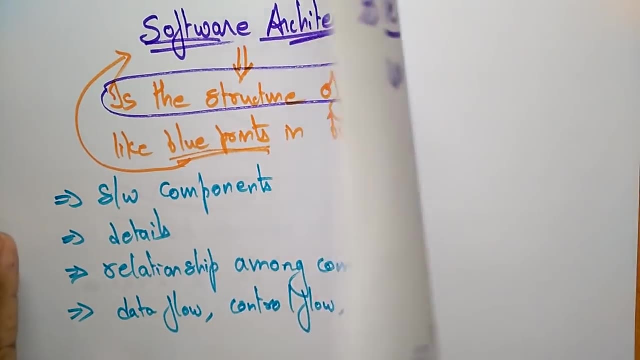 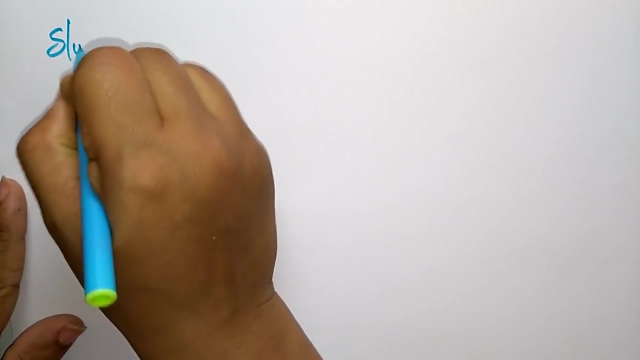 than 5,000 lines of code, then go for software architecture. okay, so only in that cases, for the larger programs only. you are going to develop a software architecture before you are starting the project, before you are writing the code for that project. okay, so let me write this software. 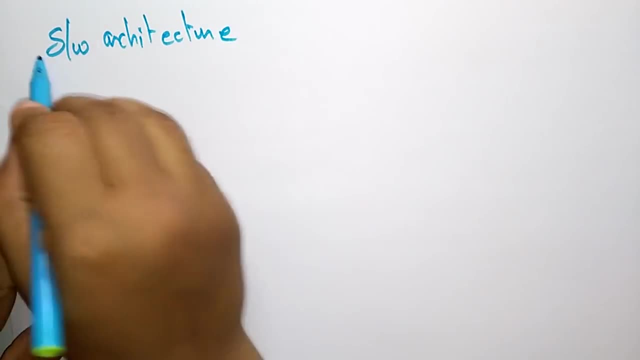 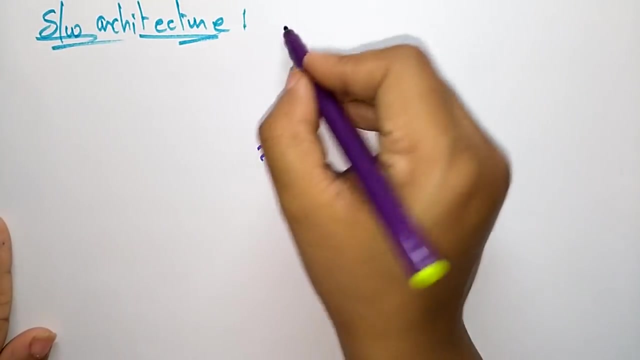 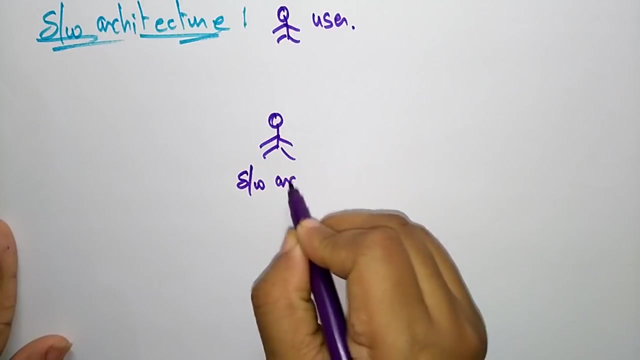 architecture nation, we can be represented in the formal diagram. so here it is. take: here the user is there user and here the software architect. so he is the person who is going to be develop the blueprint of your complete of project. so this software article, if you alsowachide or ulula wing one, we are going to develop a blueprint of your complete project. however, the software will be using these software architect. so these software architect or referencing sas will only 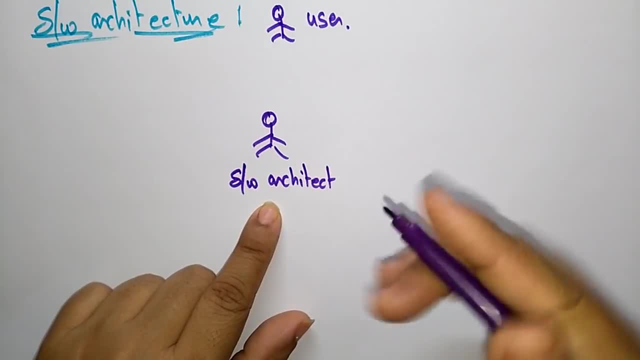 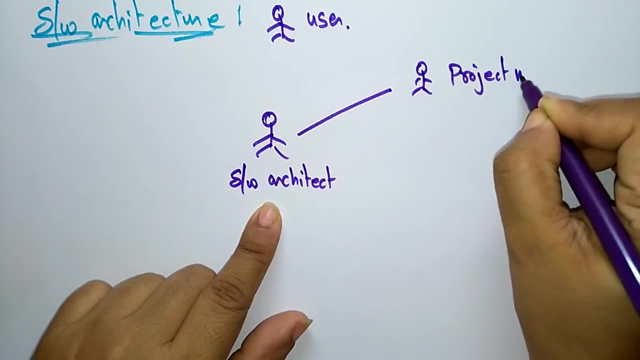 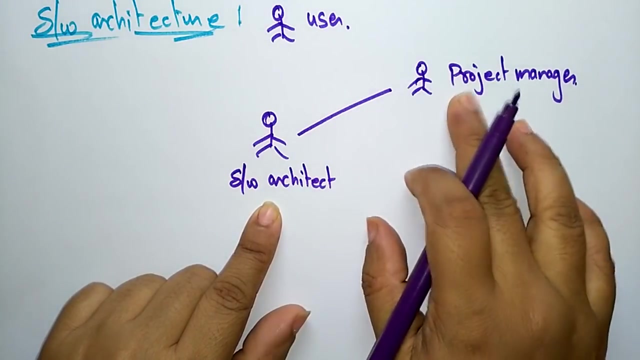 want to develop a blueprint for your software. for he has to interact with the project manager means he needs the help of project manager to gather all the requirements which are given by the customer to this manager. so the software architect has to interact with the project manager and he has to interact with the analyst. 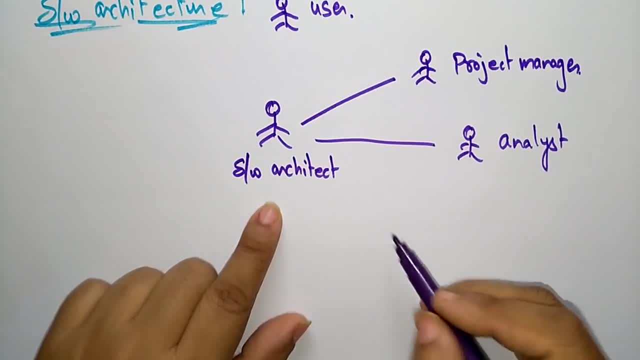 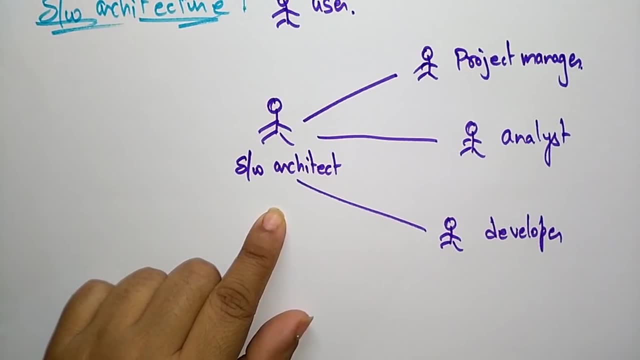 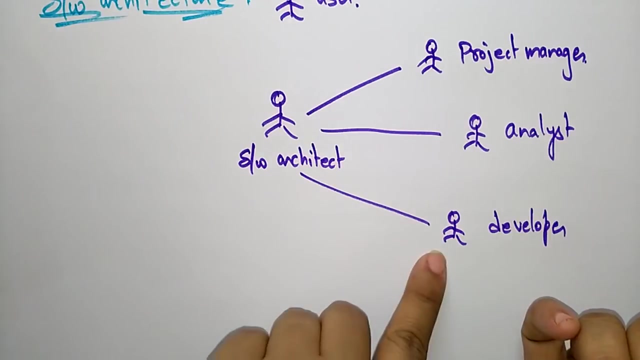 okay. at the same time, he has to interact with the developer, means which, uh, which language he is using and which components that he wants to use in the product, product or a project, so so that the software architect has interacted with the developer and he is think about the security experts also. 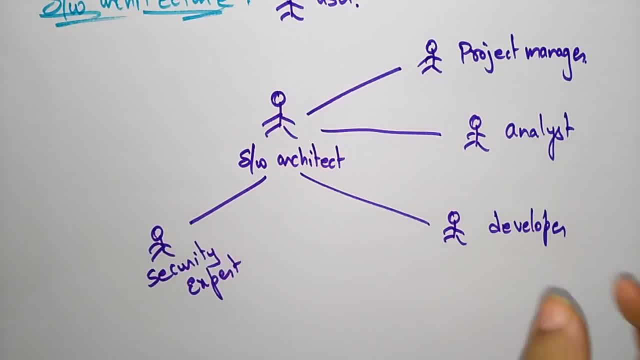 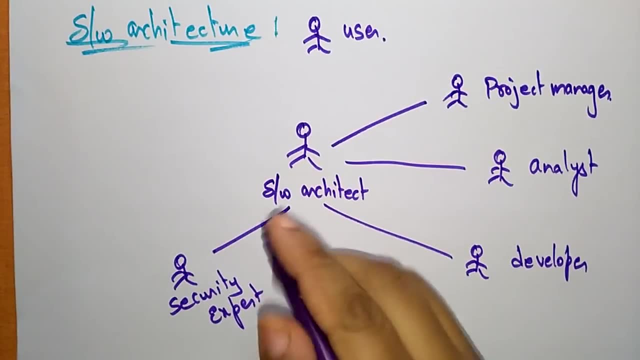 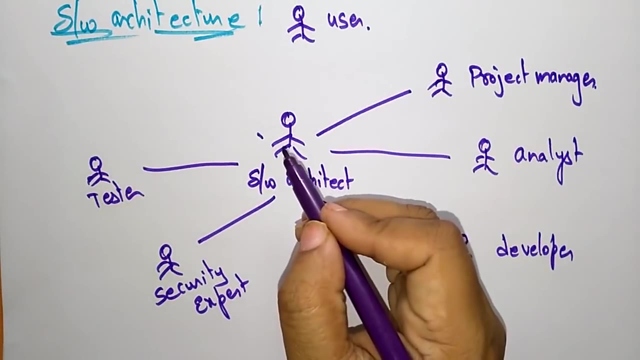 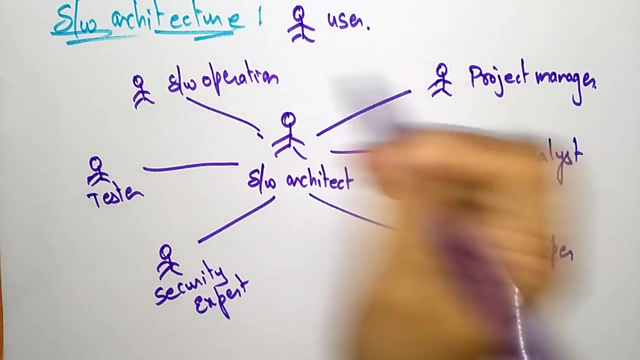 because everything should be covered in the architecture. so everything relating to the developer, analyst, security related, everything will be included in the software architecture and the tester and software operations. so, with the help of all this, the system software is going to be developed. now let us see the 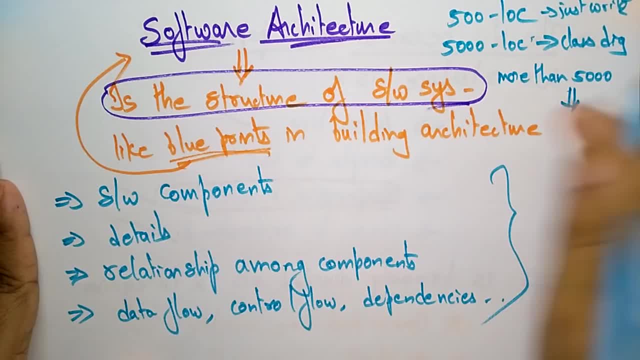 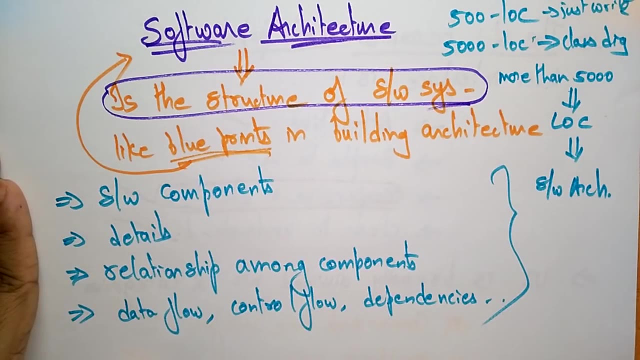 So if, in this case, if your program is more than 5000 lines of code, then go for software architecture. Okay, So only in that cases, for the larger programs only. you are going to develop a software architecture before you are starting the project. 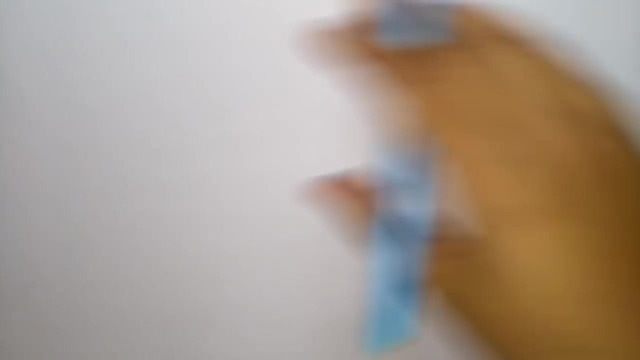 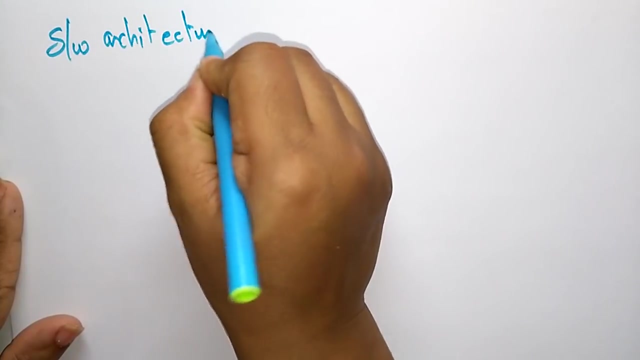 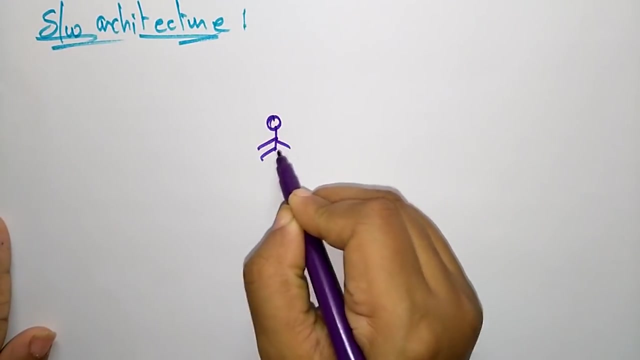 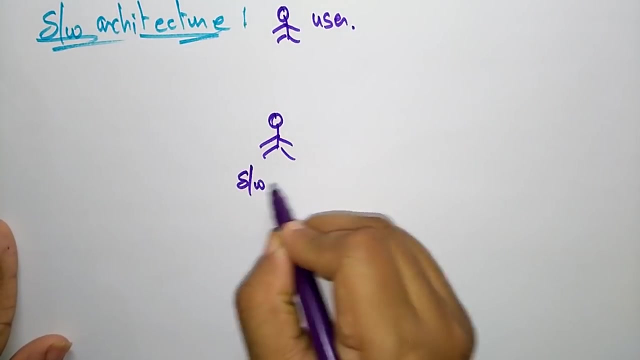 Before you are writing the code for that project. Okay, So let me write this software architecture definition So it can be represented in the form of diagram. So here let us take: here the user is there User and here the software architect. So he is the person who is going to be develop the blueprint of your complete project. 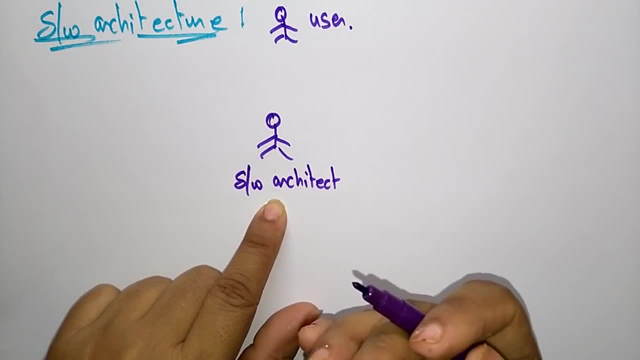 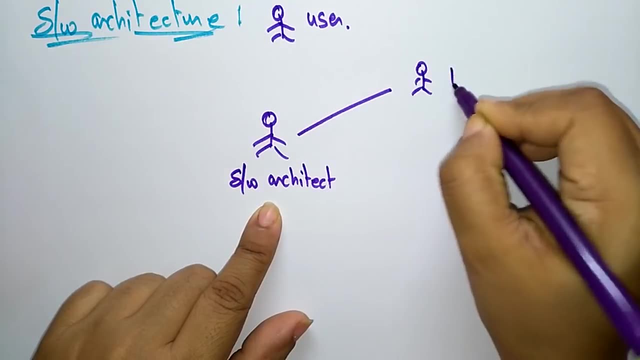 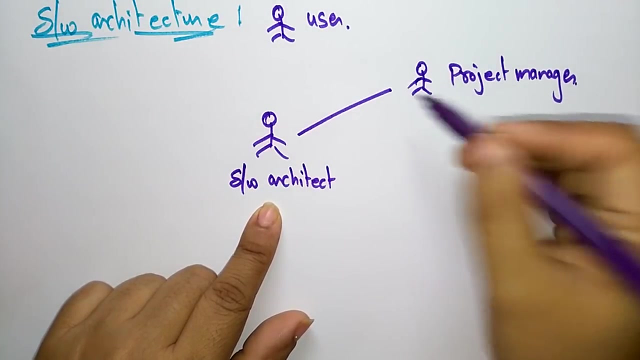 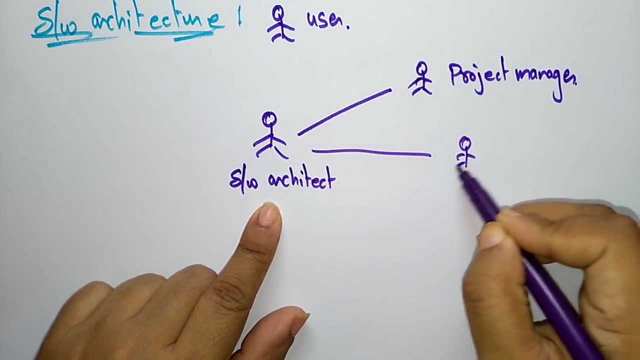 So this software architecture, If you want to develop a blueprint for your software, he has to interact with the project manager, Means he needs the help of project manager to gather all the requirements which are given by the customer to this manager. So the software architect has to interact with the project manager and he has to interact with the analyst. 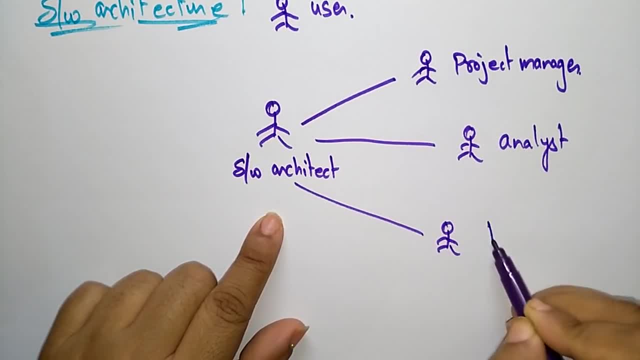 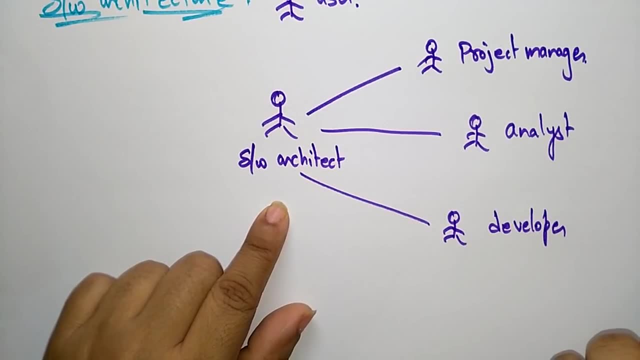 Okay. At the same time, he has to interact with the developer, means which language he is using and which components that he wants to use in the product or a project, So that the software architect has interacted with the developer and he is thinking about the security experts also. 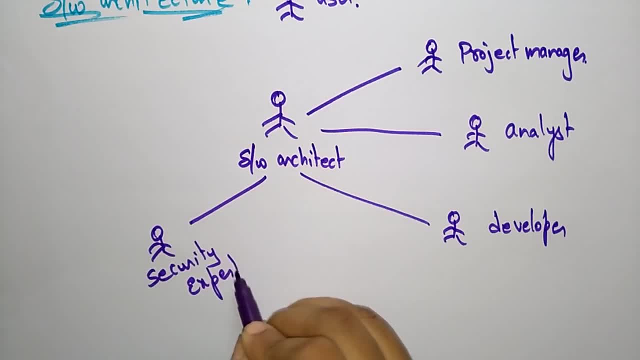 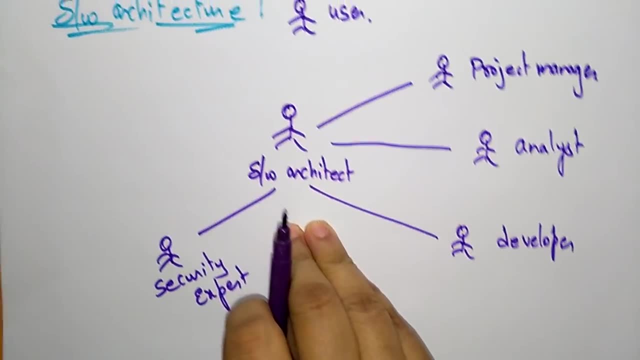 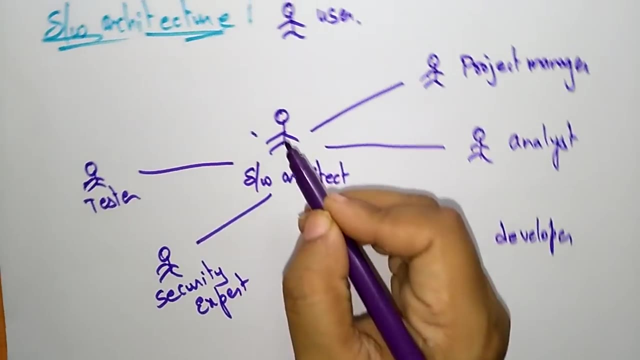 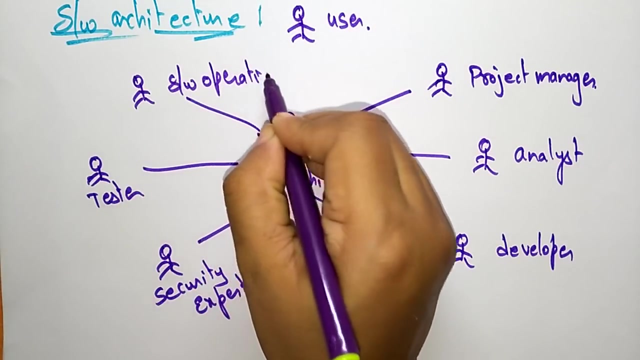 Because everything should be covered in the architecture. So everything relating to the developer, analyst, project manager, security related, Everything will be included in the architecture. Everything will be included in the software architecture And the tester and software operations. So, with the help of all this, the system software is going to be developed. 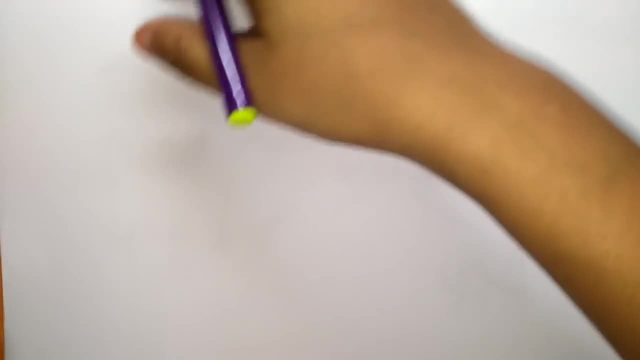 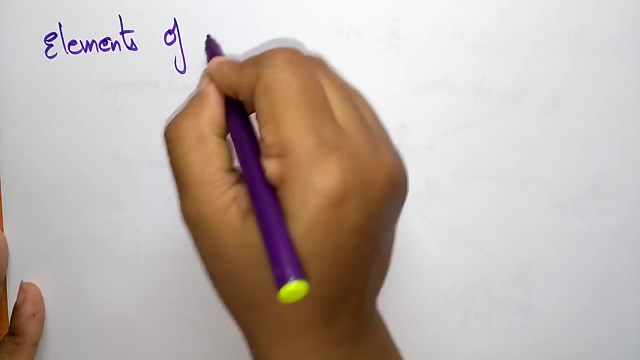 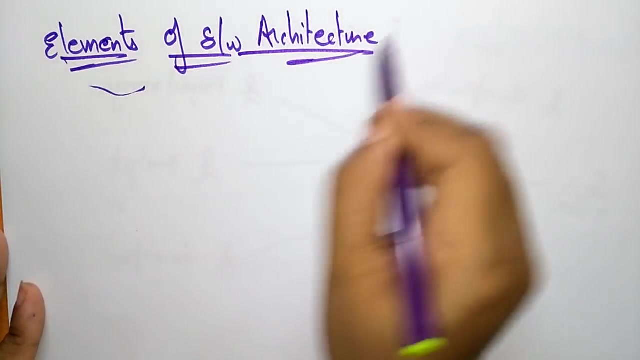 Now let us see the elements that are present in the software architecture. So what are the elements that are used in the software architecture, Elements of software architecture? So the elements that are used in the software architecture is, as usual. the first one is components. 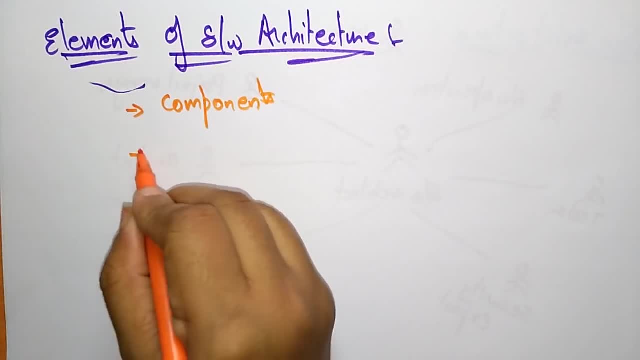 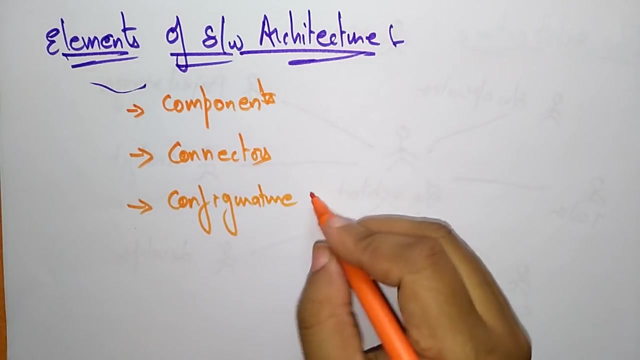 You require the components to develop a software architecture And you need the connectors to connect one component and another component, And you need the configuration topology- Means the structure Configuration, Configuration topologies, And you require system models. So these are all the different elements that are used to develop a software architecture. 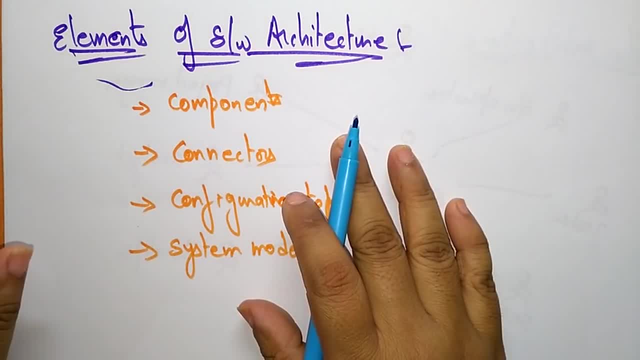 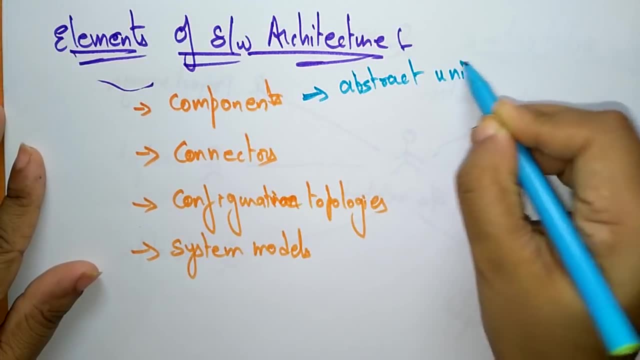 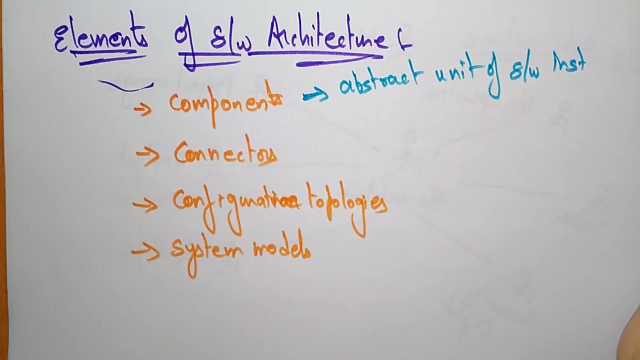 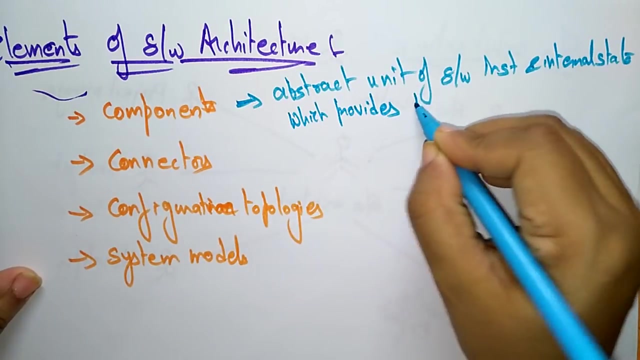 So the components is nothing, but it is an abstract unit of software instruction. It is abstract Unit of software instruction And internal state provides transformation of data. Software instruction and internal state, Internal state, which provides, Which provides transformation of data. So the main use of the components is to transform the data from. 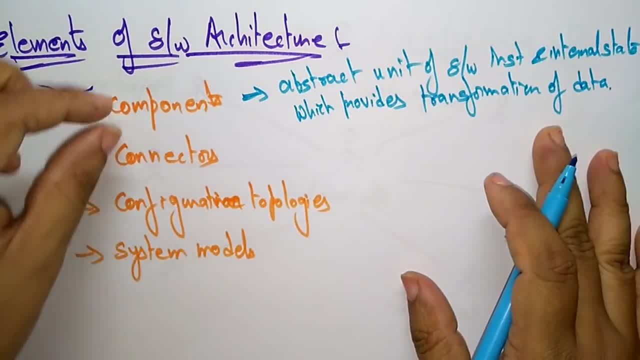 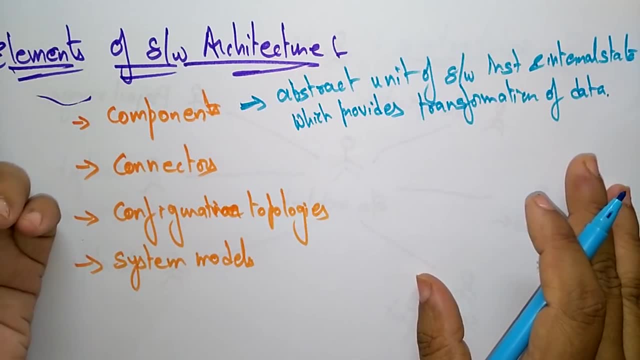 One component to another component. So this is an abstract unit. The component is an abstract unit. The module is an abstract unit. The function is an abstract unit of software instruction Which provides transformation of data, And whatever the connectors, The connectors is an abstract mechanism. 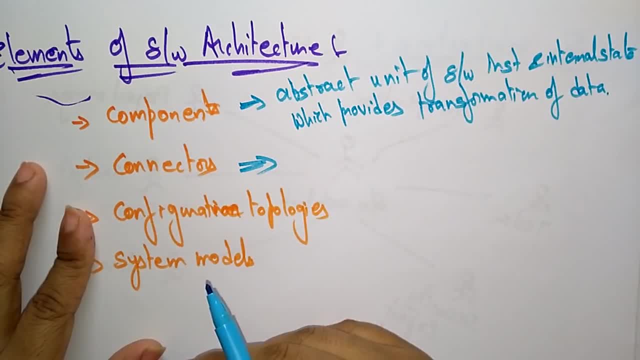 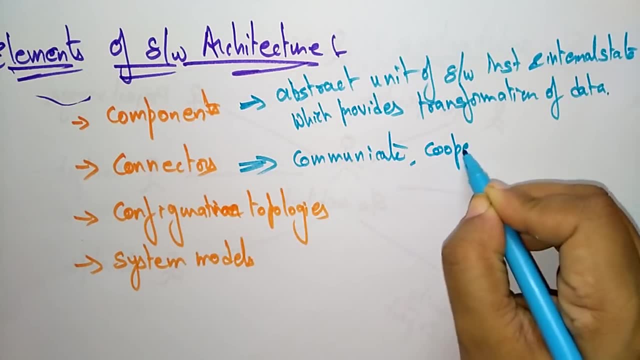 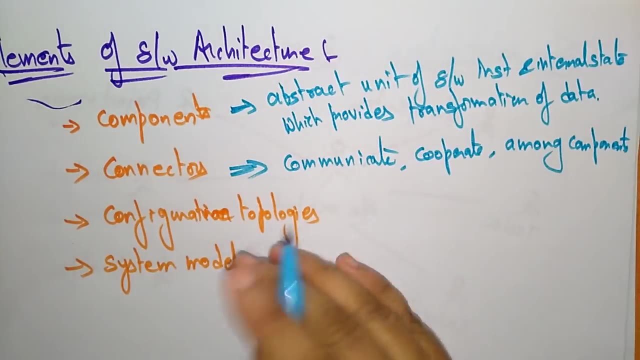 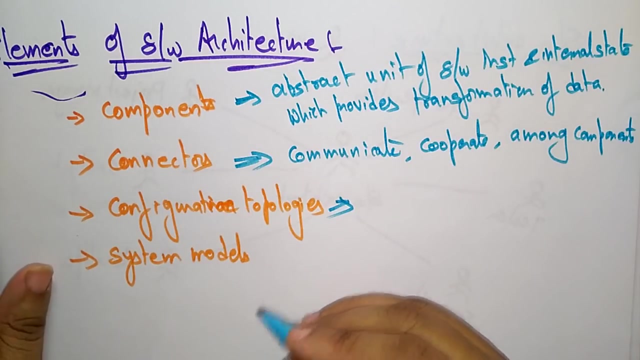 That communicates, cooperates and coordinates among the components: Communicate, Cooperate And coordinate among components. So that's about the connectors. And what about the configuration topology? A configuration topology is nothing but is a structure of architectural relationships. Structure of architectural relationships. 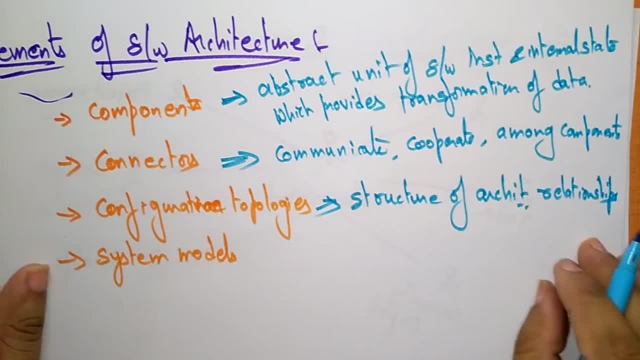 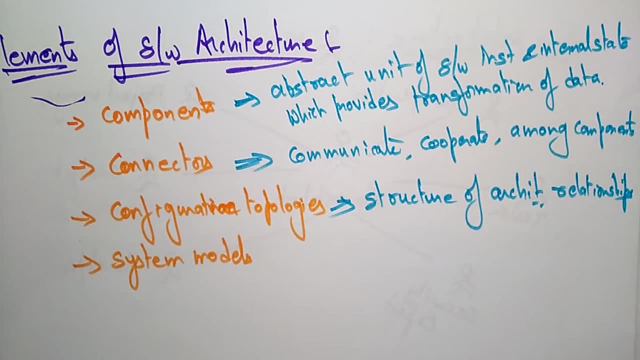 It is a structure of architectural relationships among components, Connectors- Okay- And data during a period of system runtime. So everything relating to the components, connectors and the data That is going to be communicated with the help of connectors, That will be represented in the form of structure. 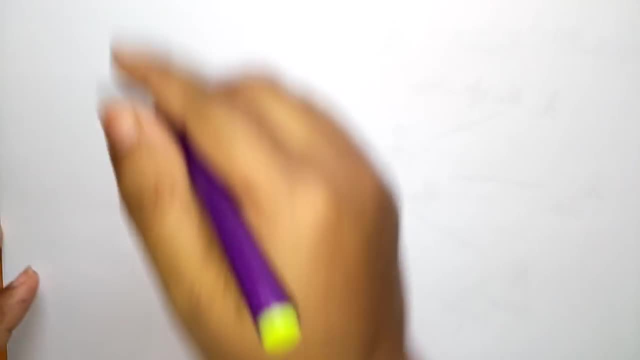 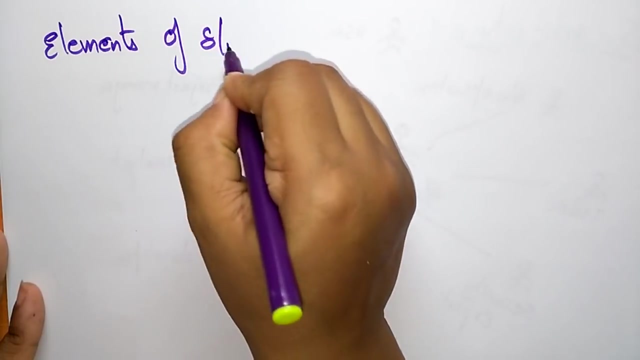 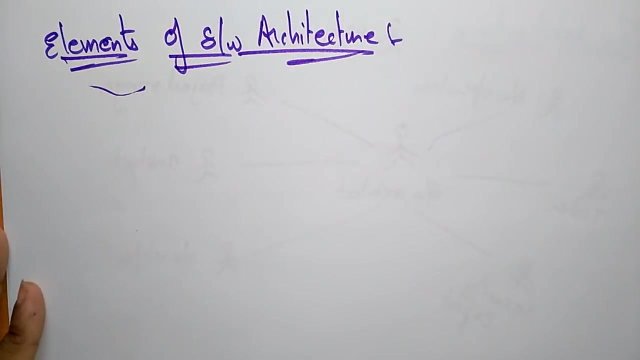 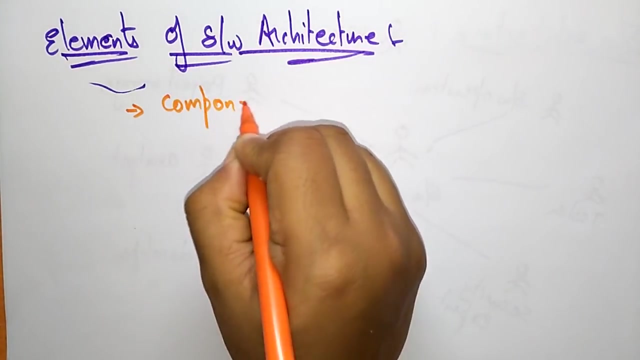 elements that are uh present in the software architecture. so what are the elements that are used in the software architecture, elements of software architecture? so the elements that are used in the software architecture is, as usual, the first ones: components. you require the components to develop a software architecture and you need the connectors. 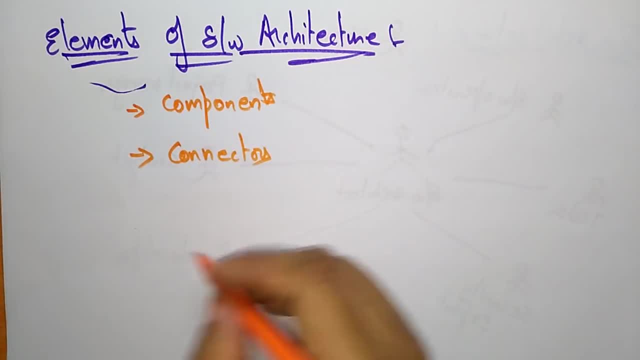 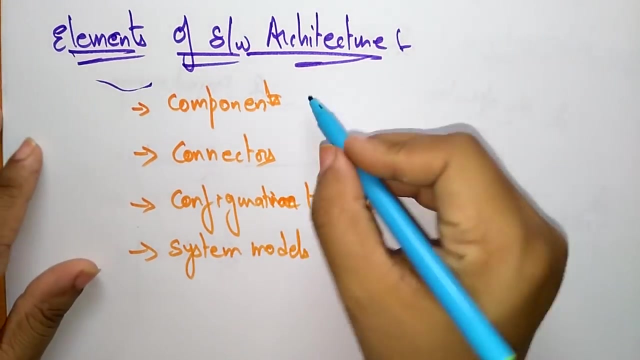 to connect one component and another component and you you need the configuration topology means the structure, configuration, configuration topologies and unique required system models. so these are all the different elements that are used to develop a software architecture. so the components is nothing, but it is an abstract unit of software instruction. it is abstract. 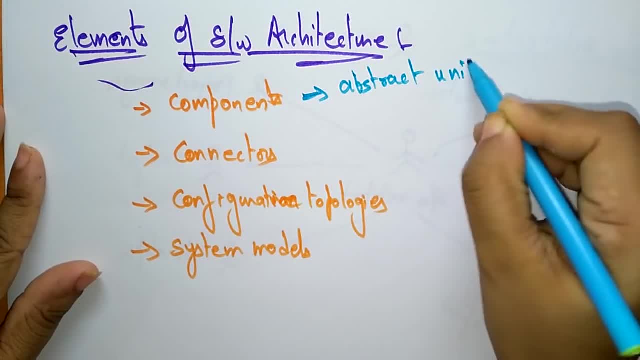 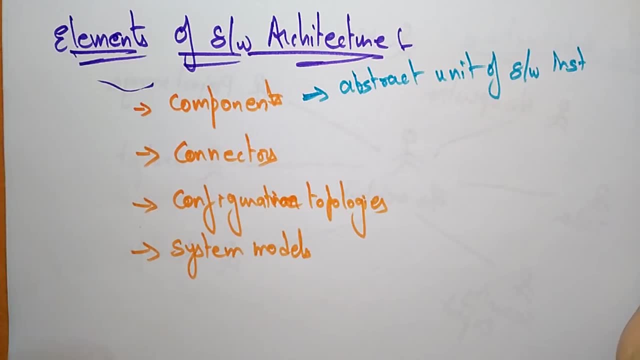 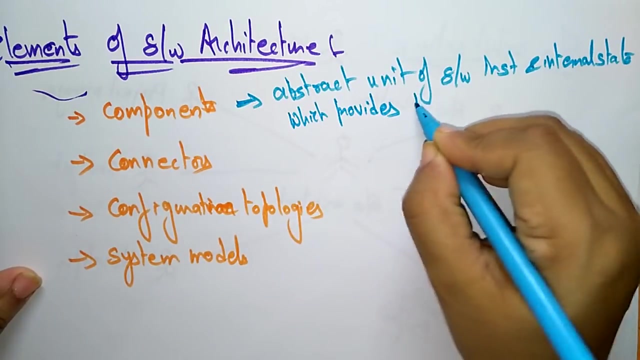 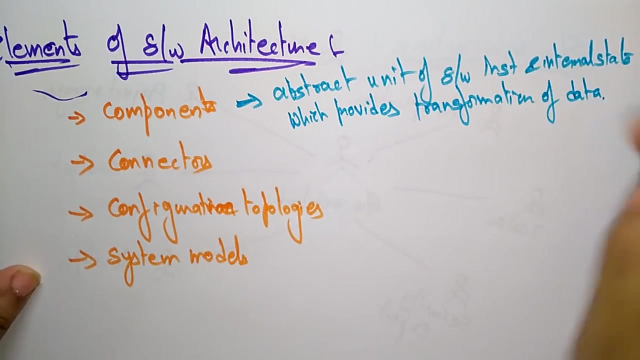 unit of software instruction and internal state provides a transformation of data. software instruction and internal state, internal state which provides, which provides transformation of data. so the main use of the components is to transform the data from one component to another component. so this is a abstract unit. the component is abstract unit. 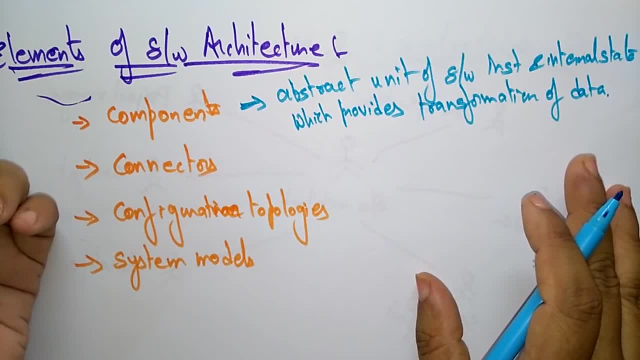 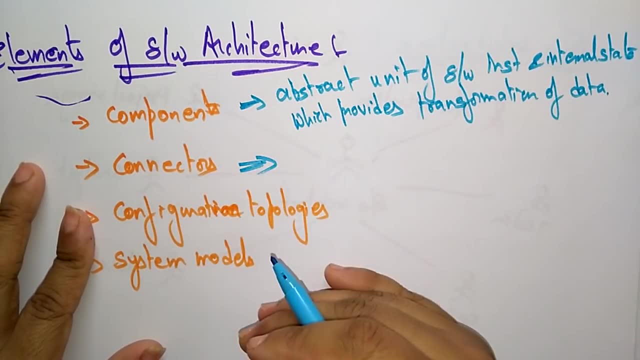 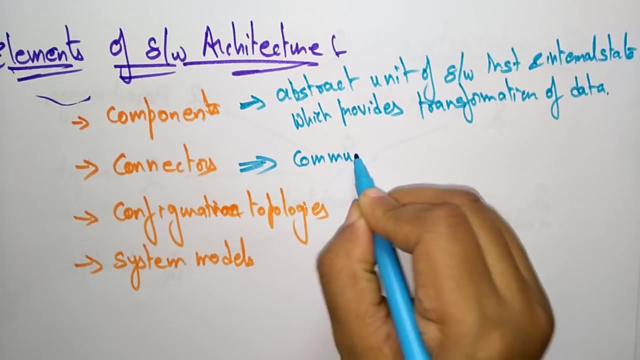 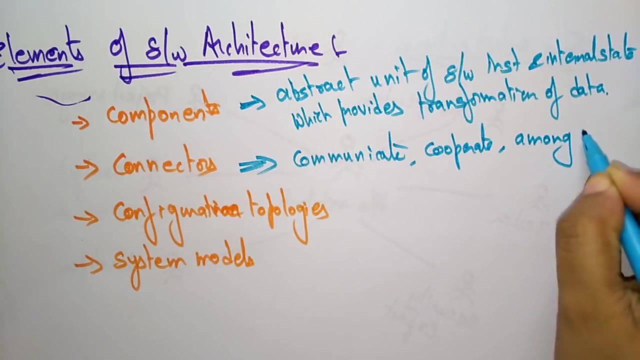 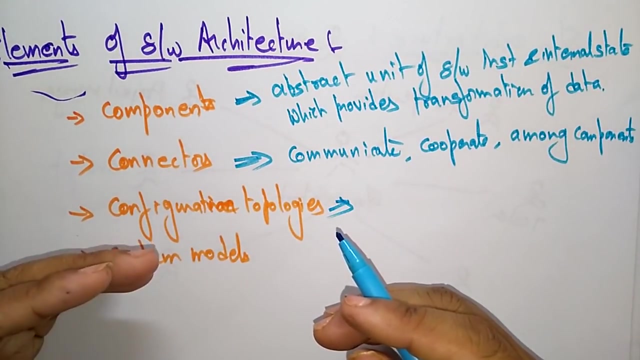 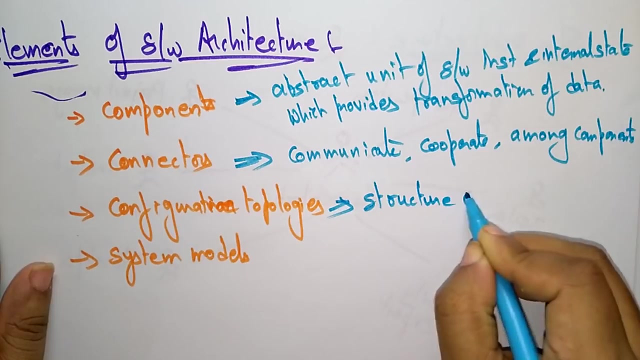 the module is an abstract unit, the function is an abstract unit of software instruction which provides transformation of data. and whatever the connectors? the connectors is abstract mechanism that communicates, cooperates and coordinates among the components communicate. so that's about the connectors and whatever the struct, orchestration topology, wow. 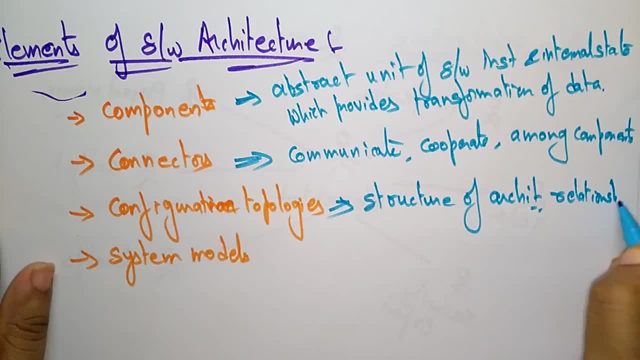 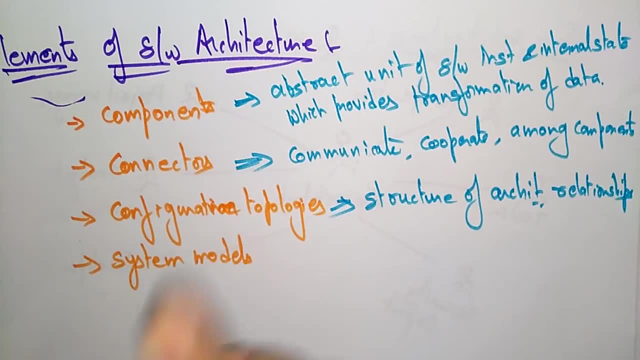 and I think I have been Gruber, formal useinken 84 and quite, ahh, steamaines, yeah, all wanted to explain that, but you can't explain that, okay, let me just explain it all first, of all of a sudden can't understand components, connectors, okay, and data during a period of system runtime, so everything relating.